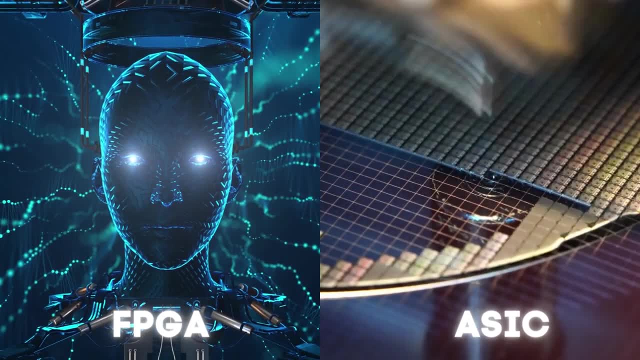 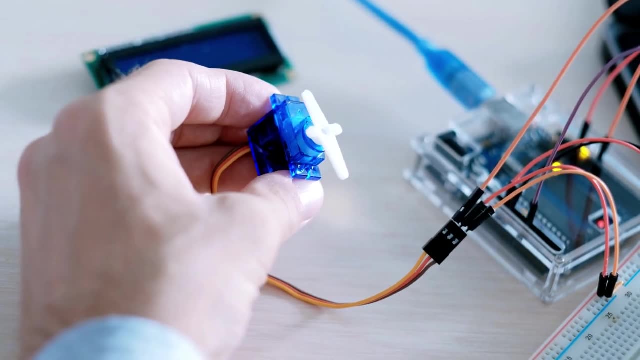 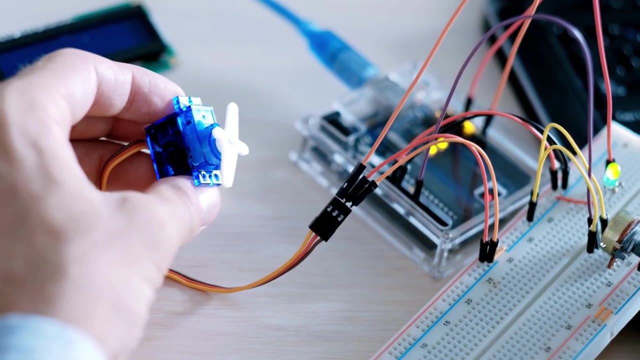 Fifth is time to market. In terms of time to market, FPGAs offer a quicker solution, as they can be reconfigured and used for different applications. For example, let's say, a lift controller had support for maximum 10 floors, but now we have a requirement of 20 floors. In this case, we can reconfigure. 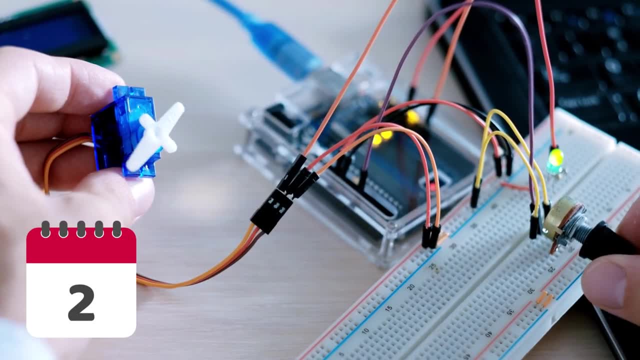 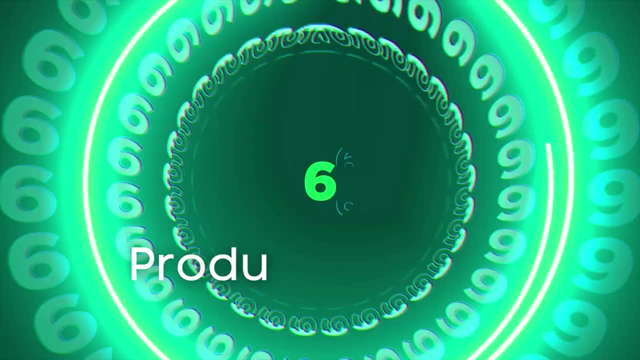 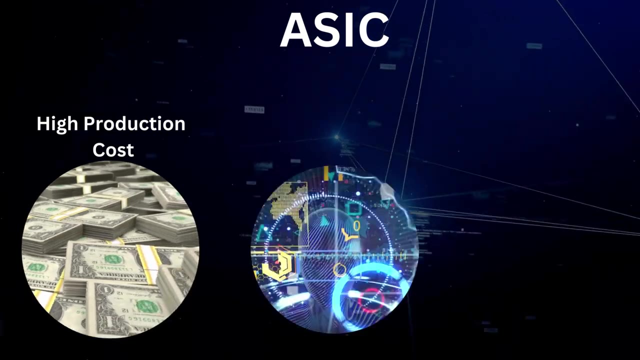 FPGA to support 20 floors within 2-3 days, while an ASIC would take months to design and manufacture. So if you are in hurry, FPGA is the winner. Sixth is production cost. ASICs is significantly higher compared to FPGAs as they are made to exact specification. 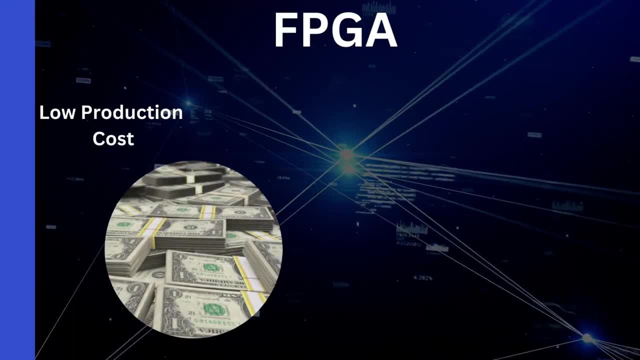 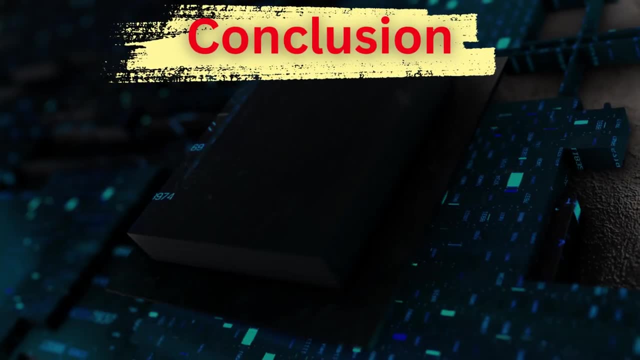 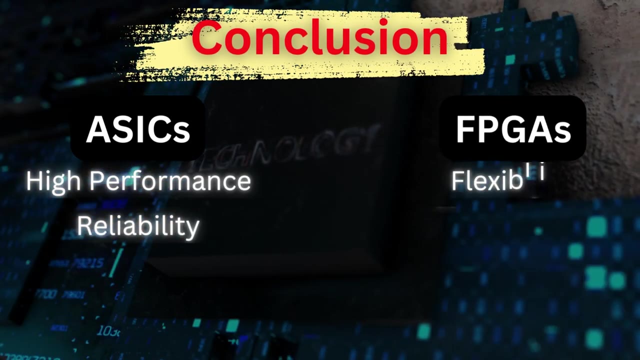 and require a more complex manufacturing process. On the other hand, FPGAs have a generic structure for all applications. Last question is which one to choose for a particular application. ASICs offer high performance and reliability for specific tasks. FPGAs offer flexibility and adaptability for multiple applications. 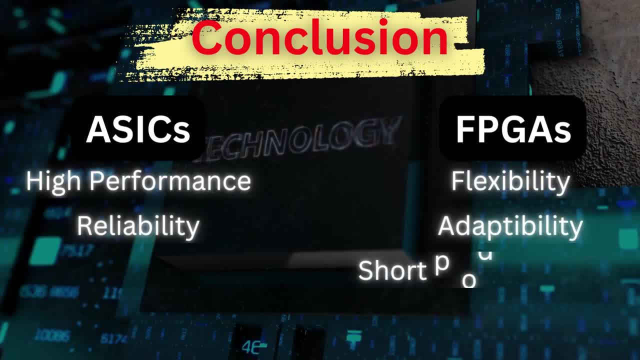 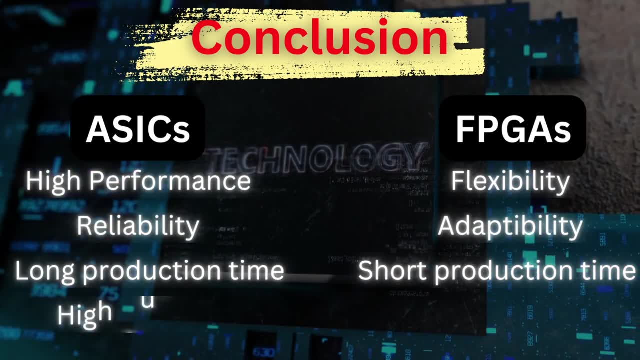 If you only have weeks time to deliver your product, choose FPGA. If you have months, ASICs is the better option. If the product require a large quantity of chips, choose ASICs. If quantity is low, then choose FPGAs. 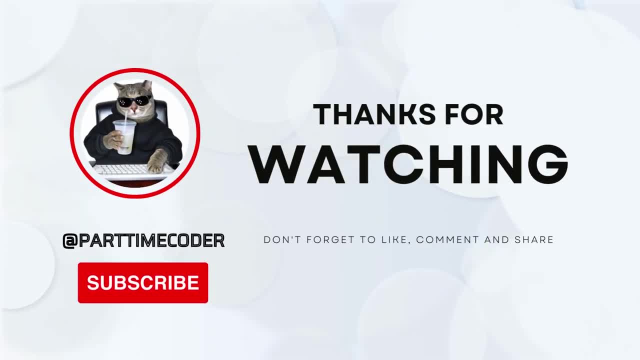 That's it for today. guys, Please like this video and subscribe to my channel. It helps me make these informative videos. 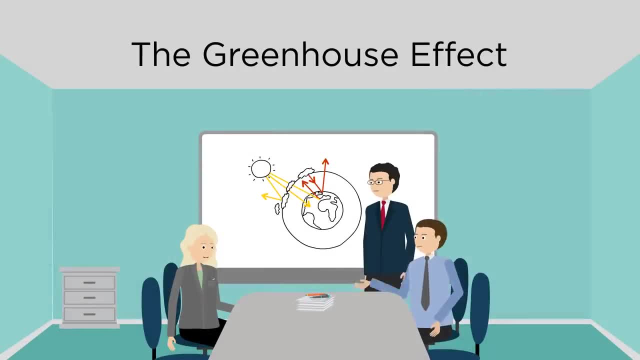 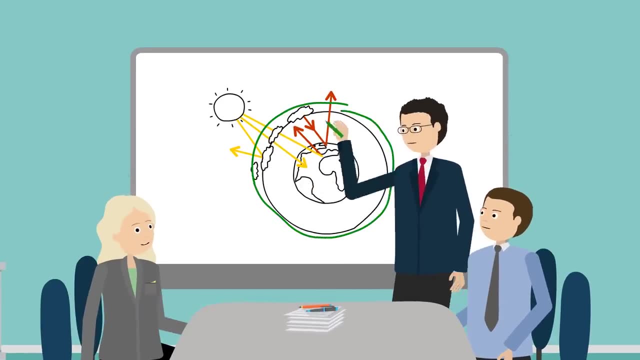 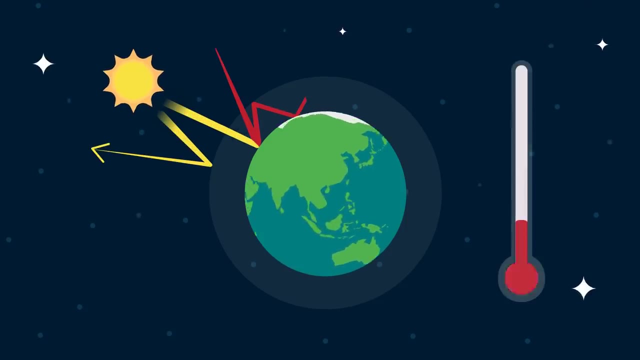 How can we describe the greenhouse effect? to make it simpler and more scientifically accurate, The common blanket model describes greenhouse gases like CO2 as a cover over the Earth. We see emitted infrared radiation bouncing back at the surface, creating a greenhouse. However, that's not the whole story. 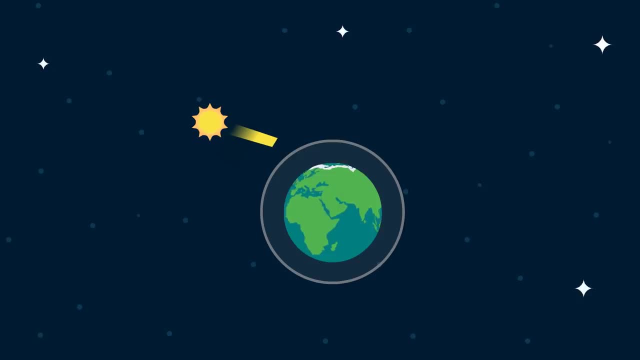 Imagine Earth's heat loss in one big bulk. The height at which Earth-submitted radiation escapes to space depends on the opacity of the atmosphere. An increase in CO2 increases the opacity, so this height increases. The lost heat depends on its temperature and the heat from the Sun. 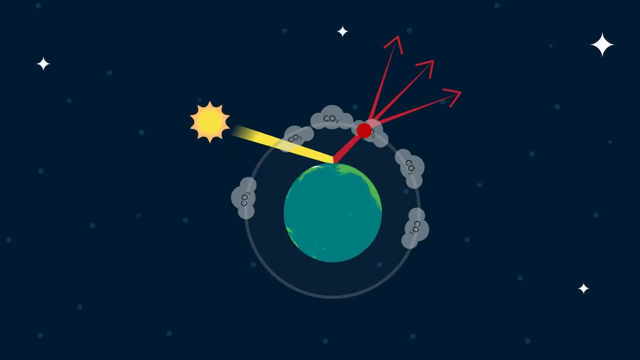 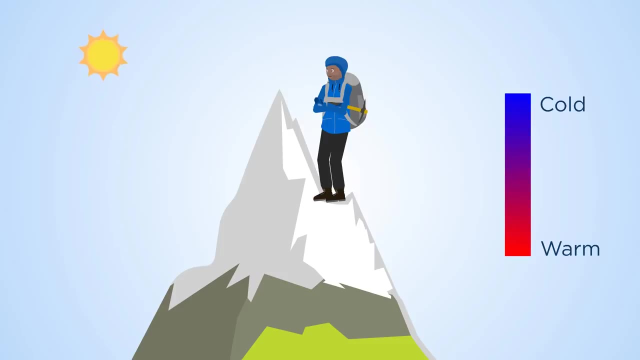 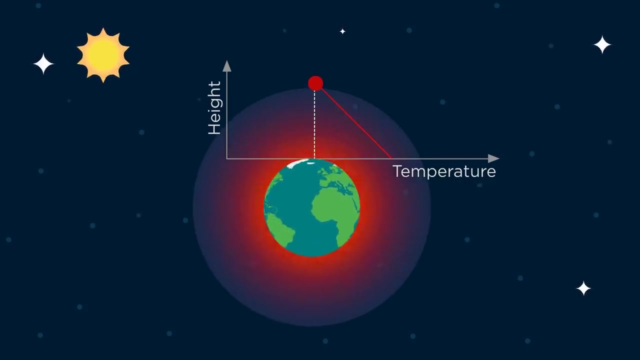 When the node rises, the surface temperature changes as determined by how the temperature varies with height. If you've climbed a mountain, you'll know it's colder at the top. Imagine stretching this temperature gradient. The area of warm air near the surface responds to the movement of the node and the temperature gradient connected to it.